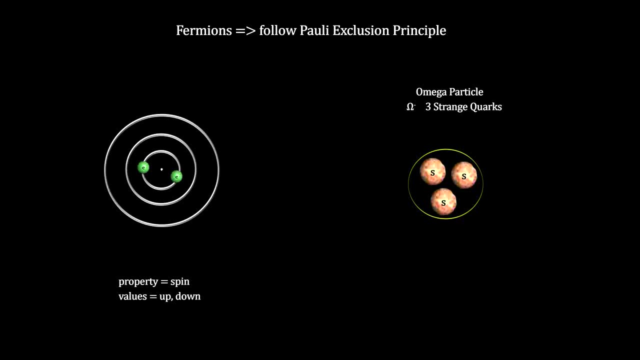 the combinations. For electrons it was spin with two values up or down. For quarks it was color charge with three values: red, blue or green. The fact that no charge has ever been seen in the mesons and hadrons made from quarks indicates 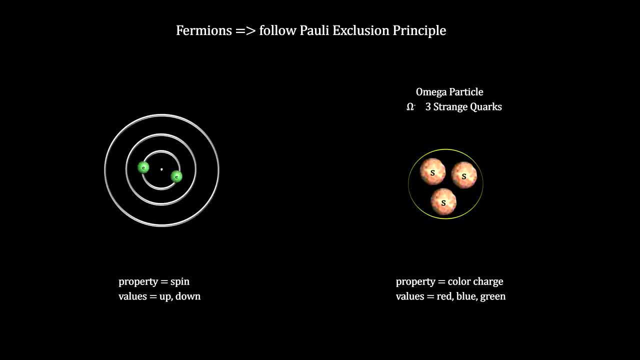 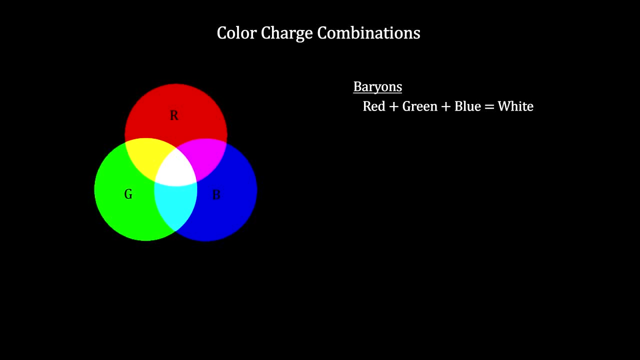 that the three charge colors neutralize each other in these configurations. This lead to the idea to use red, green and blue, because they neutralize each other when combined. Our rule for allowing quark combinations was that they had to add up to a whole unit of. 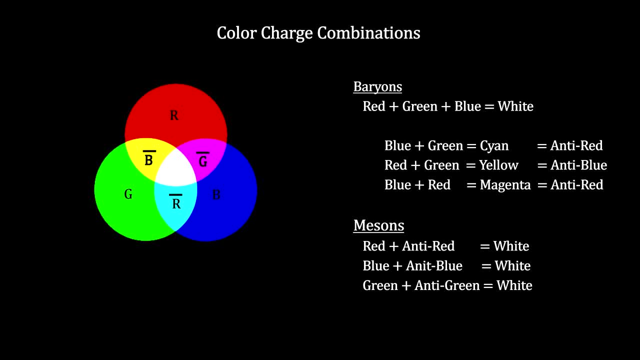 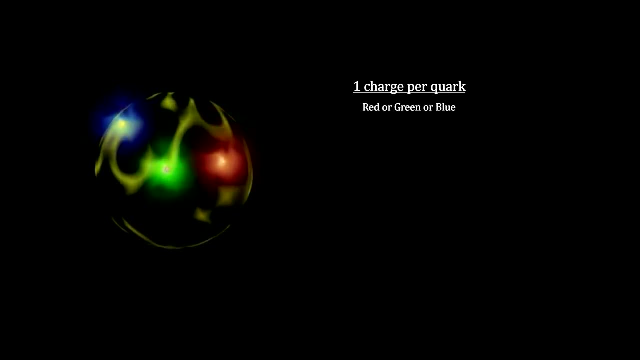 electric charge. We can now add the rule that they have to add up to no color charge at all. Another, even more dramatic difference is that gluons carry color charge as well as quarks. Where quarks carry a red, green or blue charge, gluons carry two charges: One is a color and 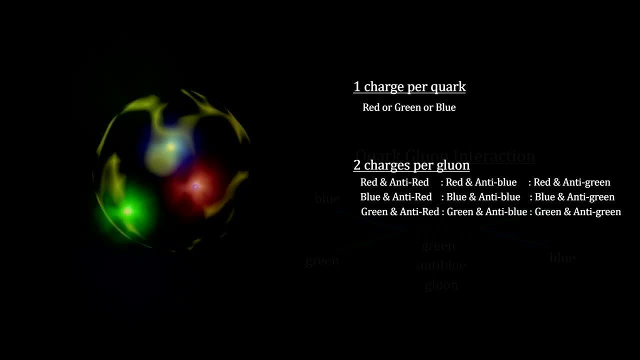 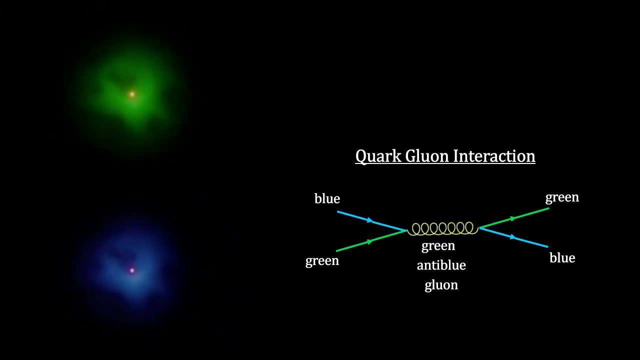 the other is an anti-color. Here's an example of how this works. We have two quarks, one with a green charge and another with a blue charge. When the green quark disturbs the gluon field, it creates a gluon. This: 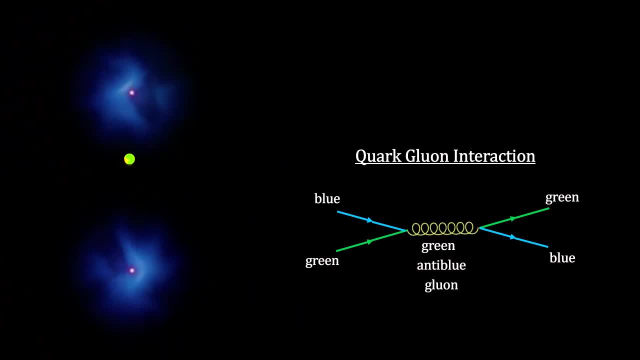 gluon carries away a green charge and an anti-blue charge. This turns the green quark blue. When the gluon encounters a blue quark, it is a blue charge. The blue quark is absorbed and the gluon's anti-blue and green charge turns the blue. 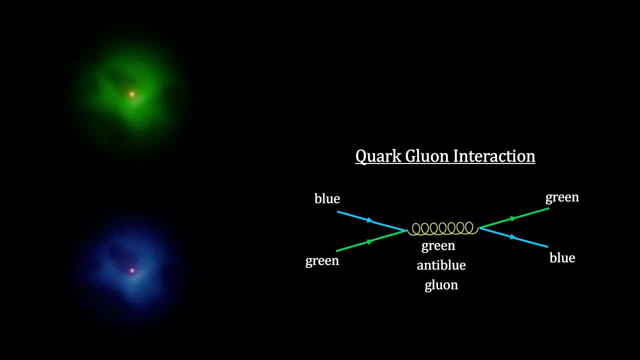 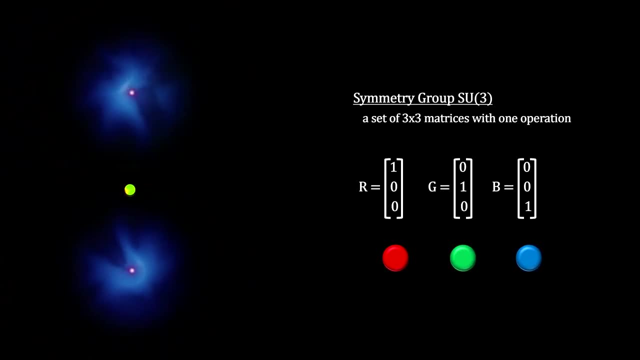 quark green. The actual functioning of the quark-gluon relationship follows the mathematical model called SU3.. The math was invented in the late 1800s and was the foundation for today's abstract algebra. A hundred years later, it turned out to be very useful for particle physics. 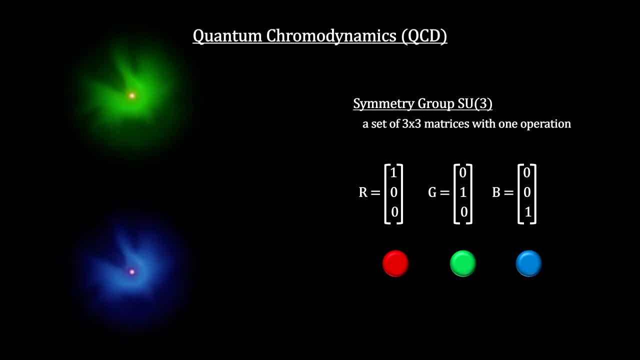 But using color is quite helpful. In fact. the study of quarks, gluons and their color charges is called Quantum Chromodynamics, or QCD for short. It is a very active area of research, and changes in our understanding are expected as we learn more.